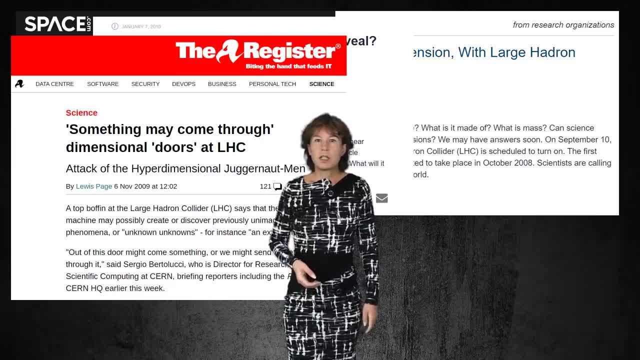 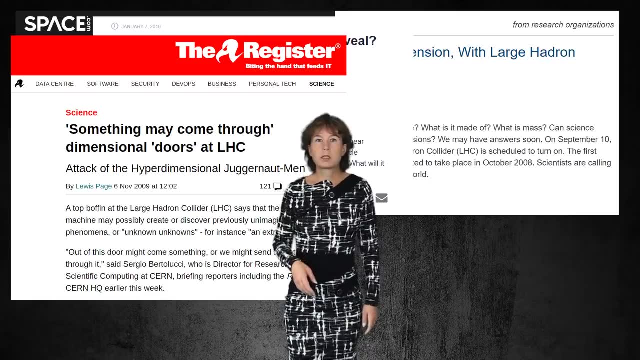 based on a hypothesis known as supersymmetry. Others talked about dark energy, additional dimensions of space, string bolts, black holes, time travel, making contact to parallel universes or unparticles, that's, particles which aren't particles. So clearly some wild ideas were in the air. 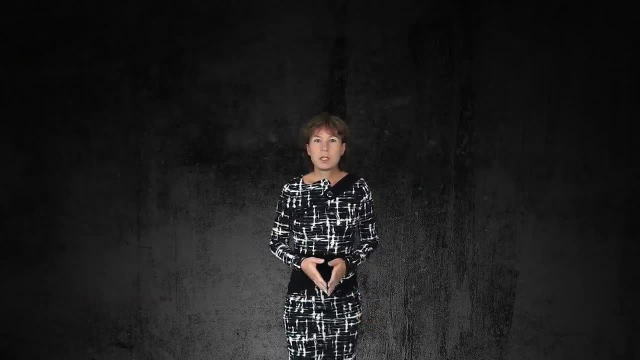 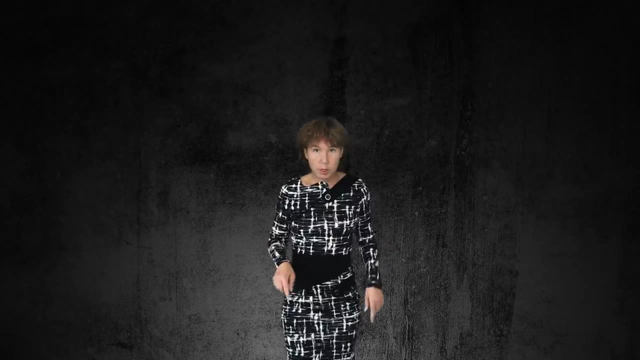 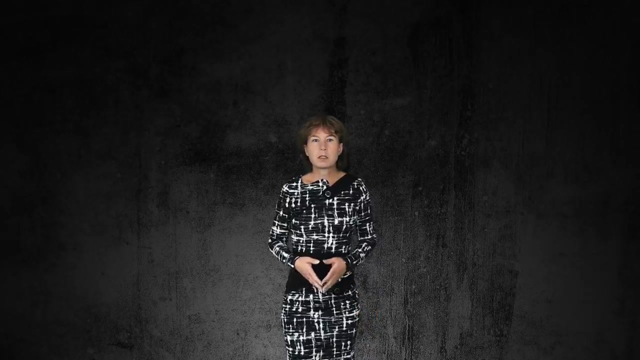 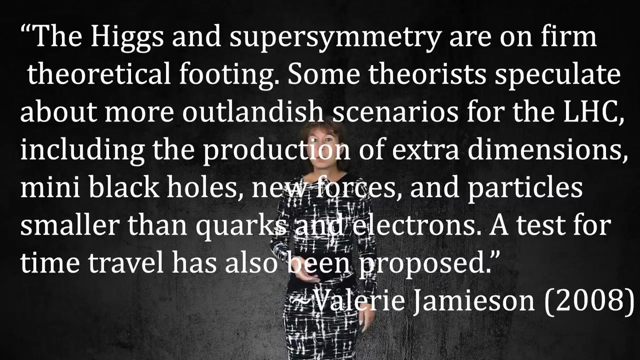 To illustrate the situation before the LHC began taking data, let me quote a few articles from back then. You find the references in the information below the video. Here's Valerie Jamieson writing for New Scientist in 2008.. The Higgs and supersymmetry are on firm theoretical footing. Some theorists speculate about more. 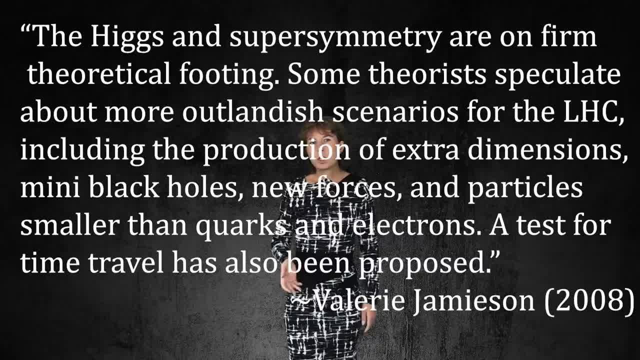 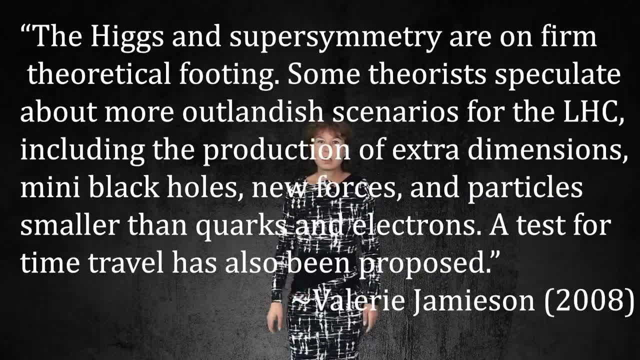 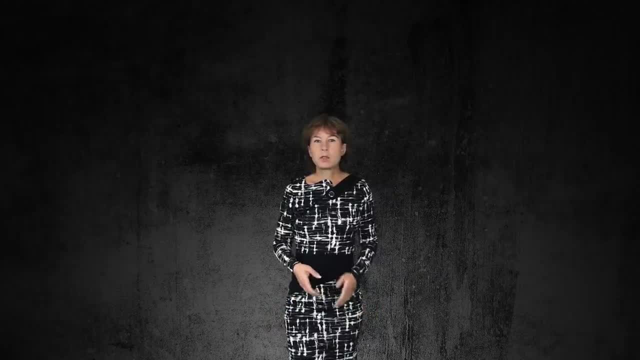 outlandish scenarios for the LHC, including the production of extra dimensions, mini black holes, new forces and particles smaller than quarks and electrons. A test for time travel has also been proposed. Or here's Ian Sample writing for the Guardian, also in 2008.. Scientists have some pretty good. 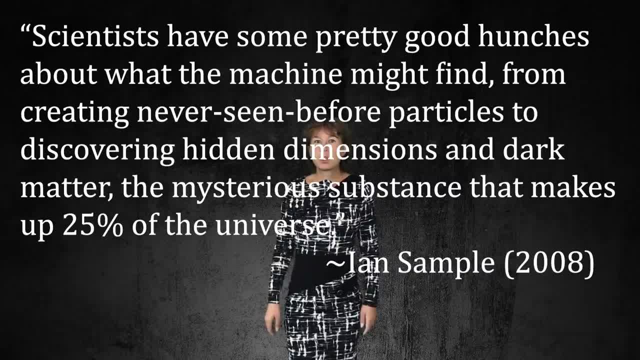 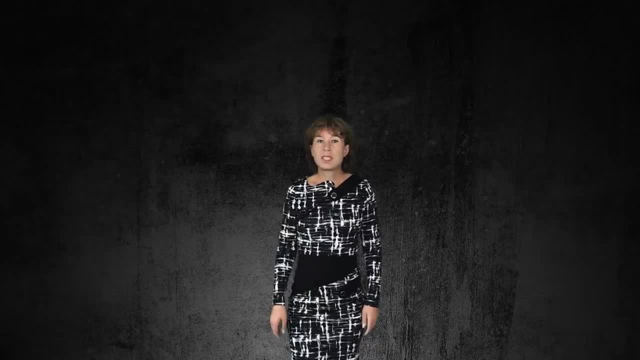 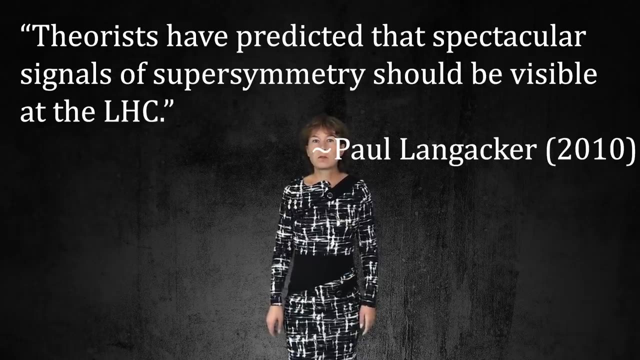 hunches about what the machine might find, from creating never-seen-before particles to discovering hidden objects. Here's Paul Langacker in 2010, writing for the APS. Theorists have predicted that spectacular signals of supersymmetry should be visible. 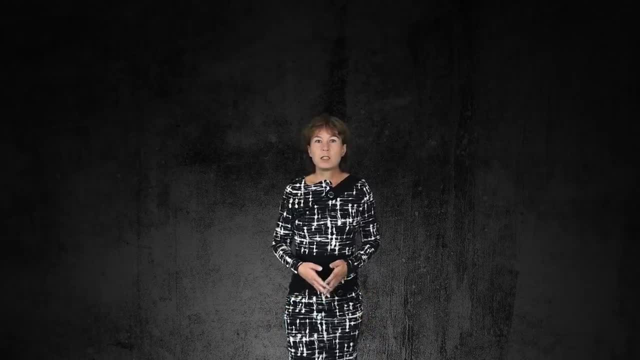 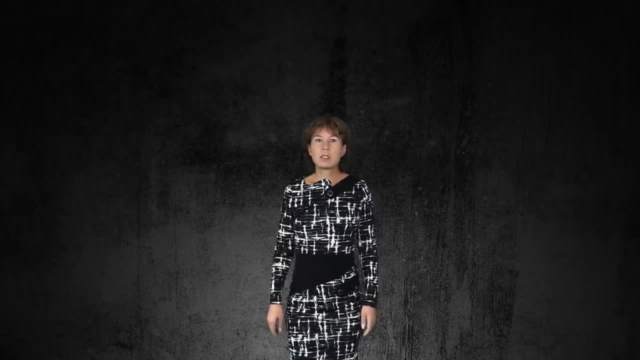 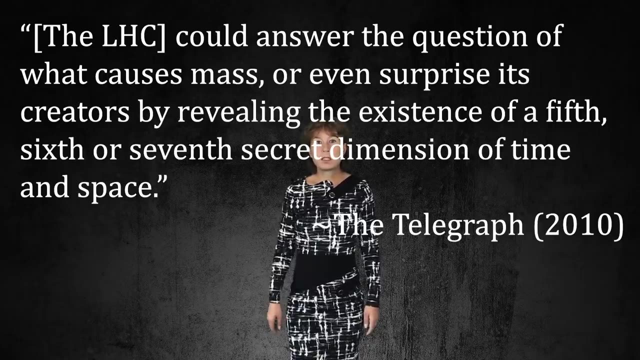 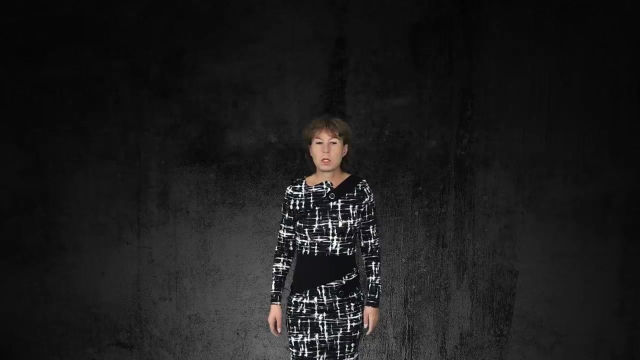 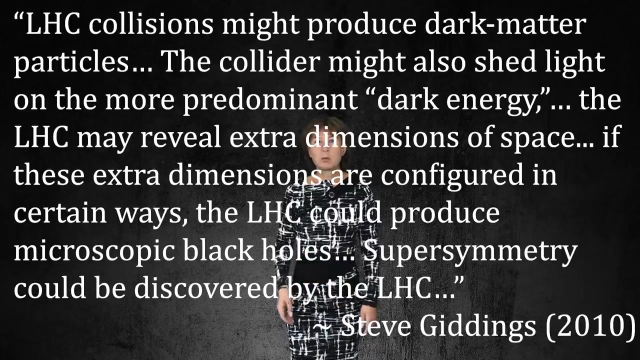 entirely The Telegraph in 2010,. The LHC could answer the question of what causes mass, or even surprise its creators by revealing the existence of a fifth, sixth or seventh secret dimension of time and space. One final one: here's Steve Giddings writing in 2010 for Phys Org. LHC collisions might. 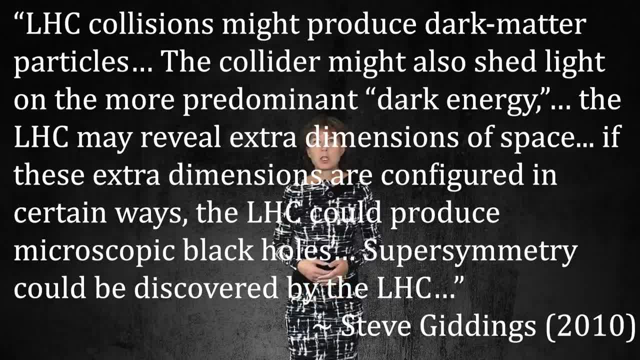 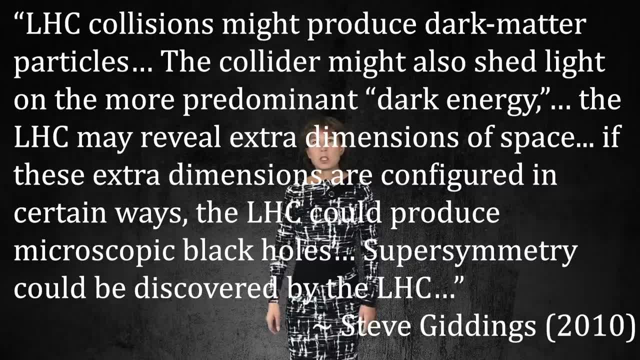 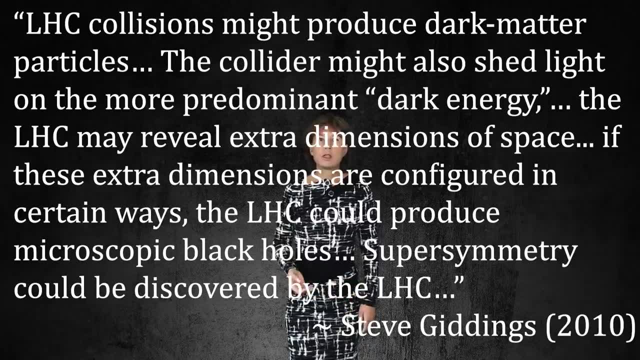 produce dark matter particles. The collider might also shed light on the more predominant dark energy. The LHC may reveal extra dimensions of space. If these extra dimensions are configured in certain ways, the LHC could produce microscopic black holes. Supersymmetry could be discovered by the LHC. 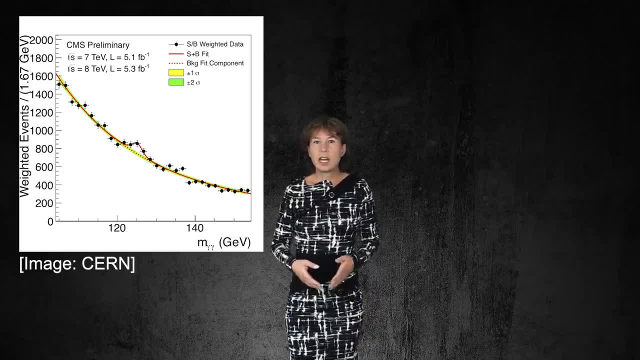 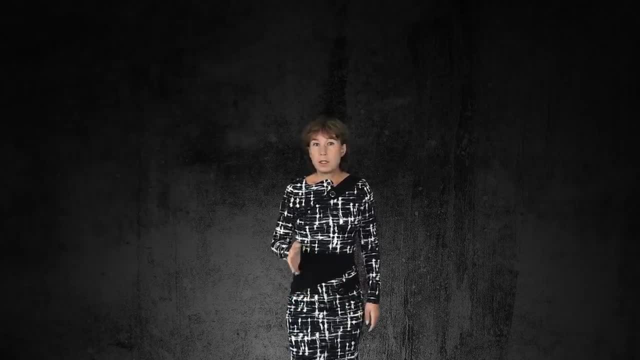 The Large Hadron Collider has been running since 2010.. It has found the Higgs boson, But why didn't it find any of the other things? This question is surprisingly easy to answer. There was never good reason to expect any of these things in the first place. 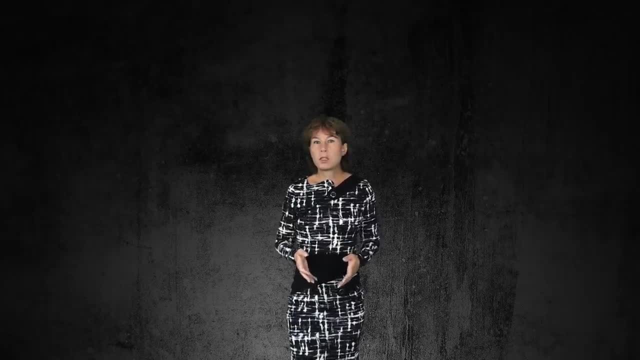 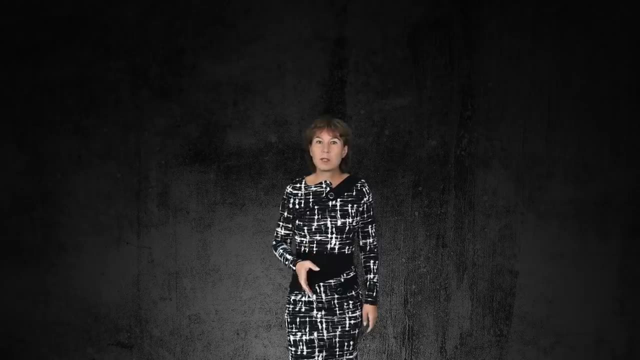 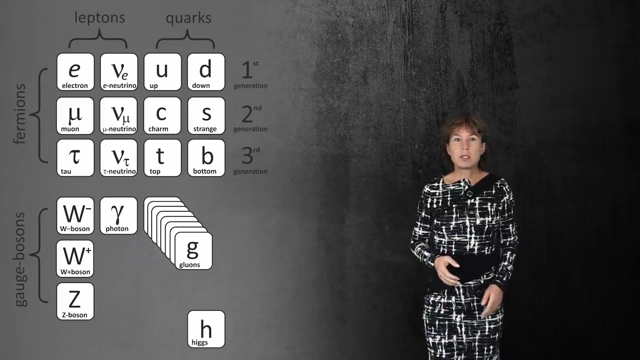 The more difficult question is: why did so many particle physicists think that those were reasonable expectations, and why has not a single one of them told us what they have learned from their failed predictions? To see what happened here, it is useful to look at the difference between the prediction. 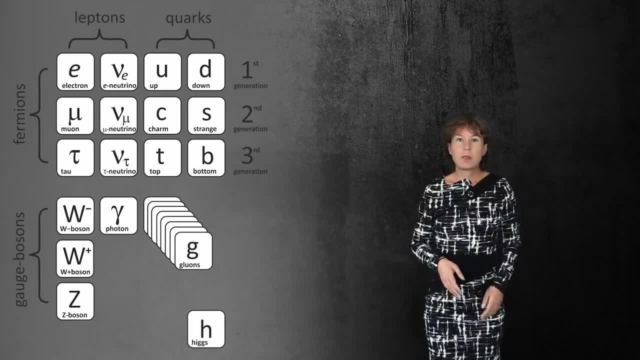 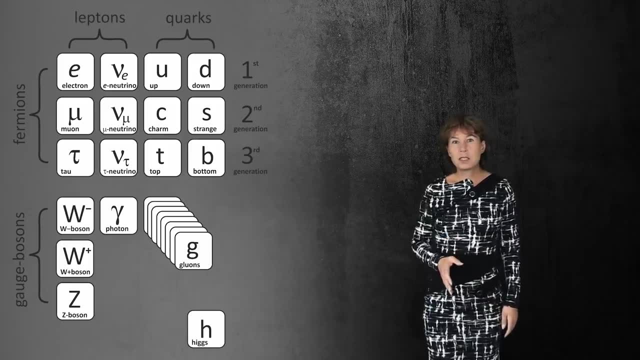 of the Higgs boson and the other speculations. Let's start with the Higgs boson. The standard model without the Higgs does not work properly. It becomes mathematically inconsistent at energies that the LHC is able to reach. Concretely, without the Higgs, it predicts probabilities larger than one, which makes no sense. We therefore knew, before the LHC turned on, that something new had to happen. It could have been something else besides the Higgs. The Higgs was one way to fix the problem with the standard model. But there are other ways. However, the Higgs turned out to be right. All other proposed ideas- extra-dimensions, supersymmetry, time travel and so on- are unnecessary. These theories have been constructed so that they are compatible with all existing observations. 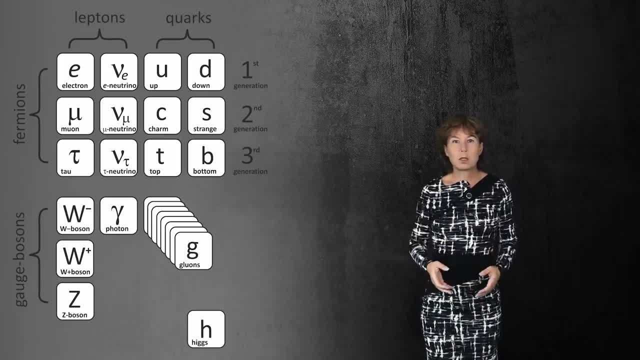 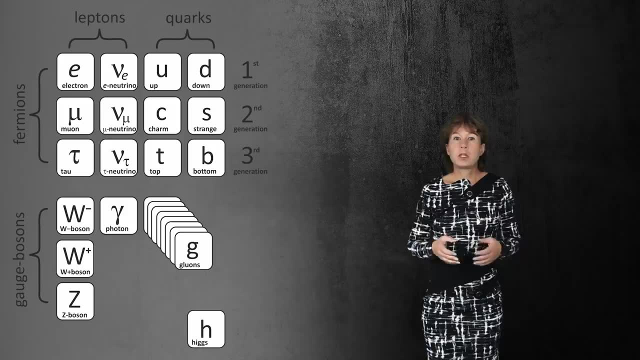 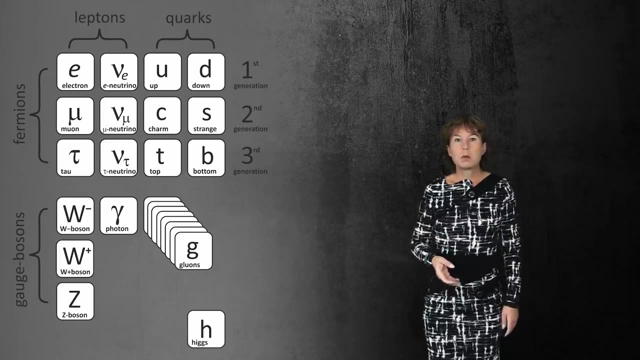 but they are not necessary to solve any problems with the standard model. They are basically wishful thinking. The reason that many particle physicists believed in these speculations was to establish a future for the Higgs boson, a different one. speculations is that they mistakenly thought the Standard Model has another problem, which 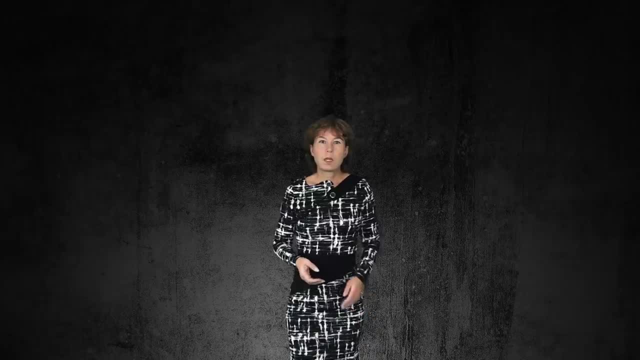 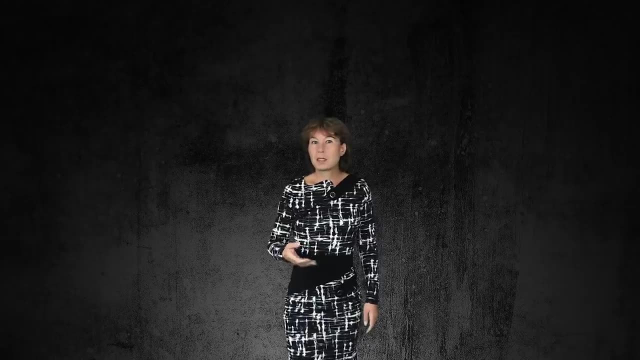 the existence of the Higgs would not fix. I am afraid that many of them still believe this. This supposed problem is that the Standard Model is not technically natural. This means the Standard Model contains one number that is small, but there is no explanation for why this number is small. 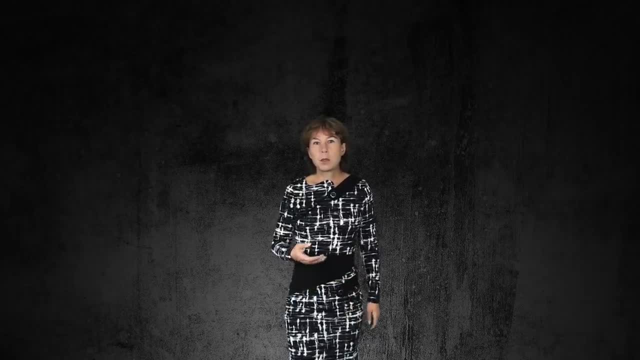 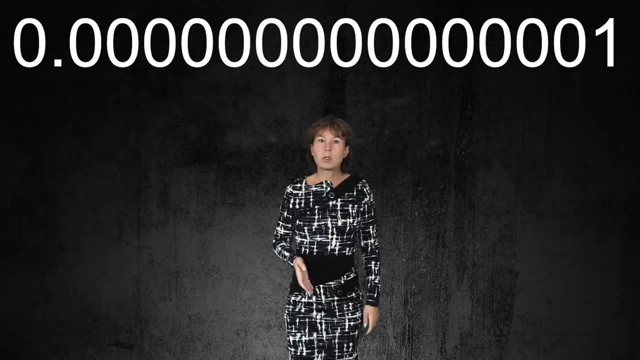 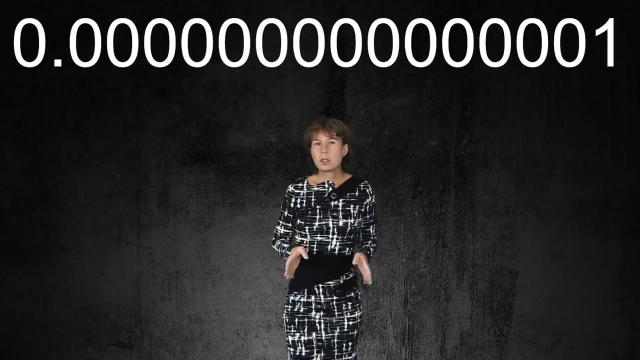 This number is the mass of the Higgs boson divided by the Planck mass, which happens to be about 10 to the minus 15.. The Standard Model works just fine with that number and it fits the data. But a small number like this, without explanation, is ugly and particle physicists didn't want to.